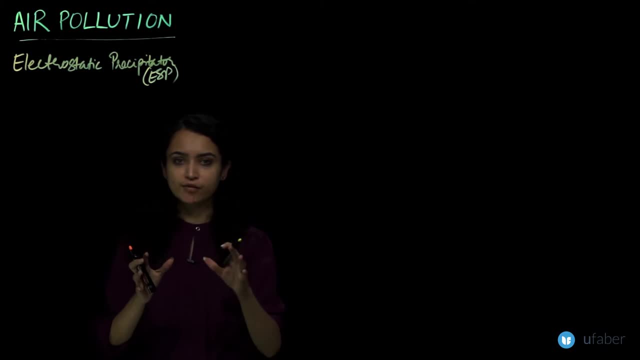 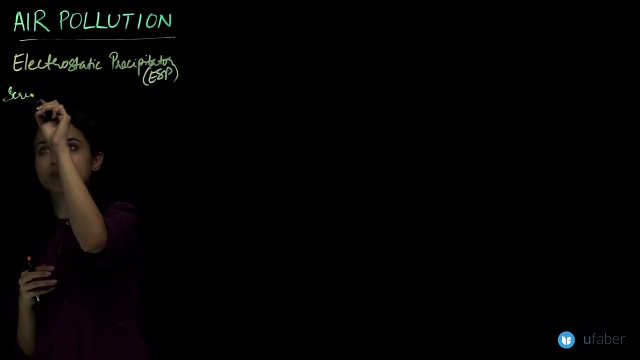 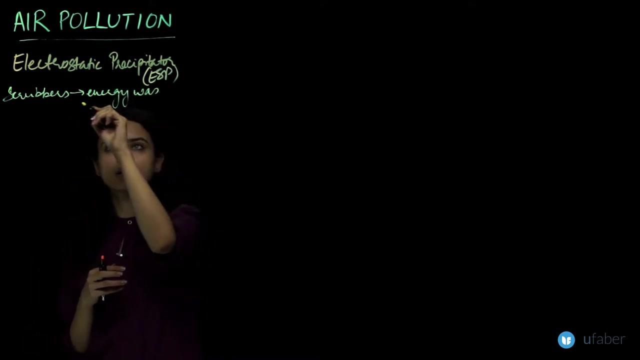 energy when we were supplying water. So in energy that we were applying was to the entire media, and so in the scrubbers, energy was applied to the entire media, while in the ESP water was nice, one can apply water to the entire cell. 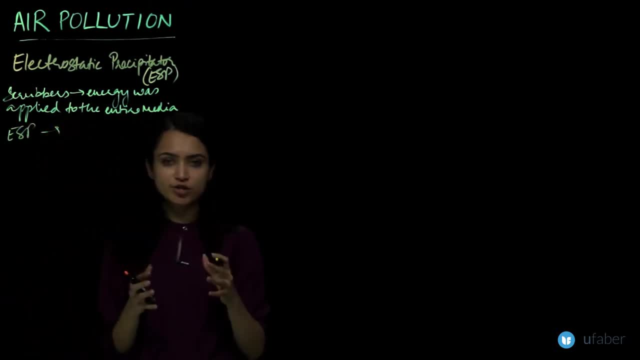 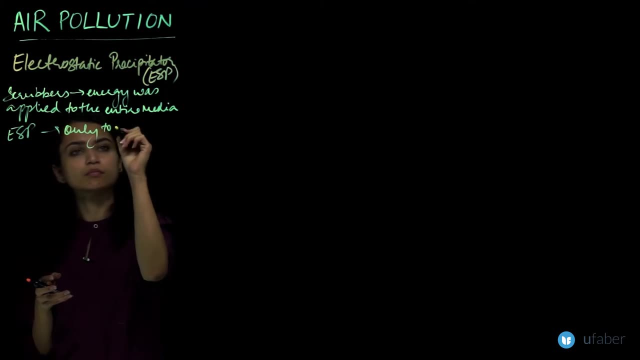 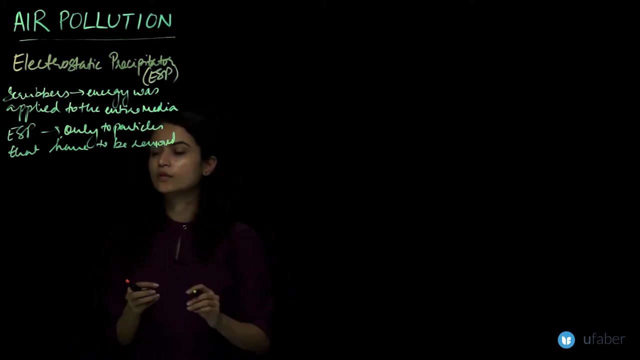 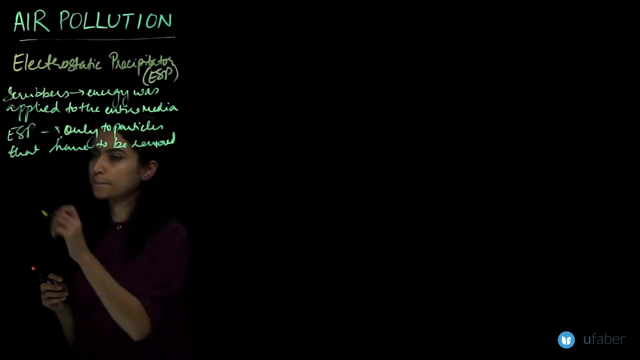 Yeah, Yeah, definitely, Exactly. The energy is only applied to the particles that have to be removed. So the energy is only applied to the particles that has to be removed. Here, therefore, I am not saying less energy is required, but we can remove finer particles. 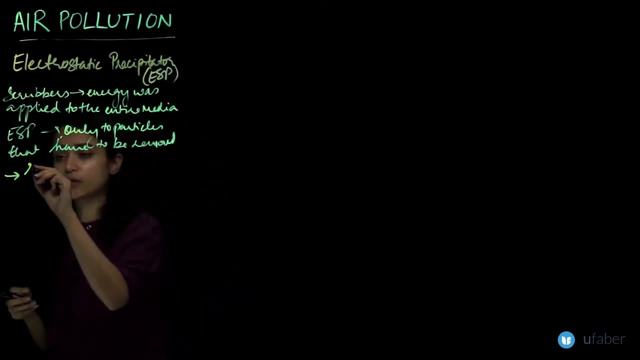 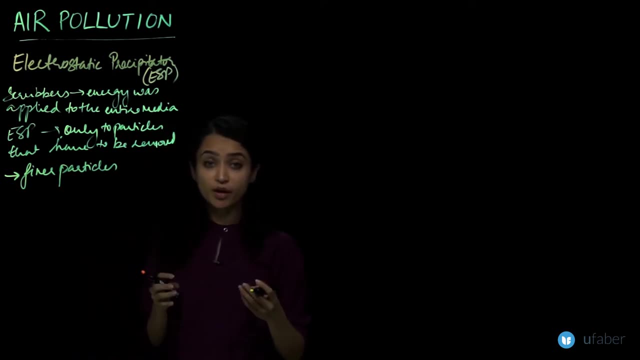 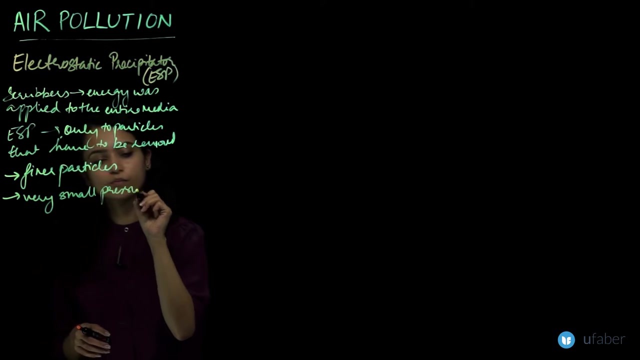 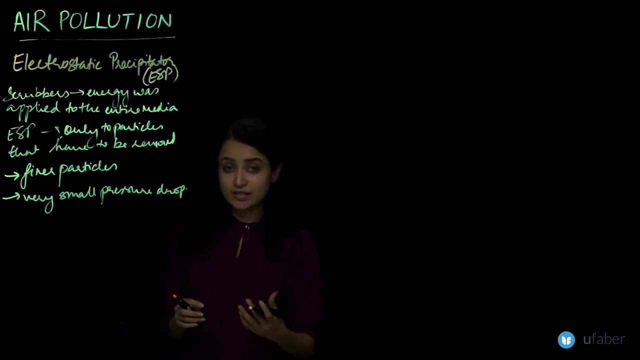 than were covered even with scrubbers, So we can remove finer particles. There is no pressure drop, so you can directly move from an ESP to the next instrument and expect some good results. How an ESP works is explained in three steps. Before I begin with the three steps, I think I will draw a diagram so that it's easy to. 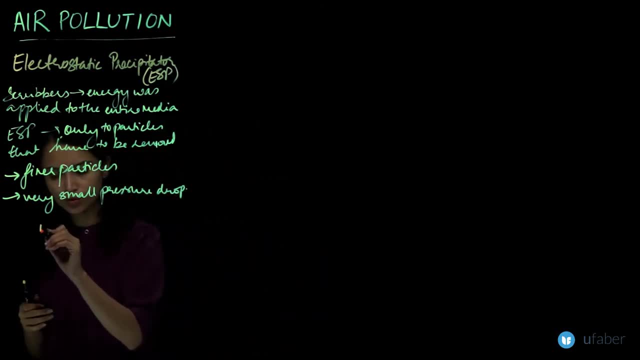 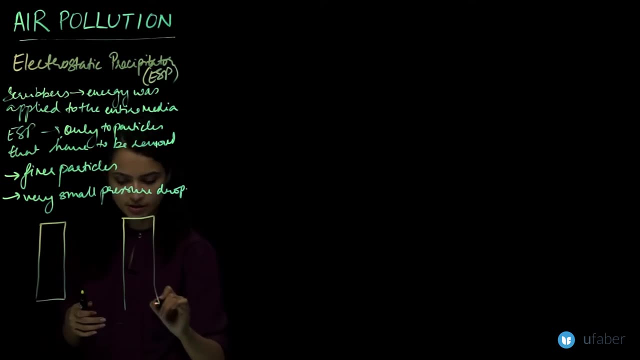 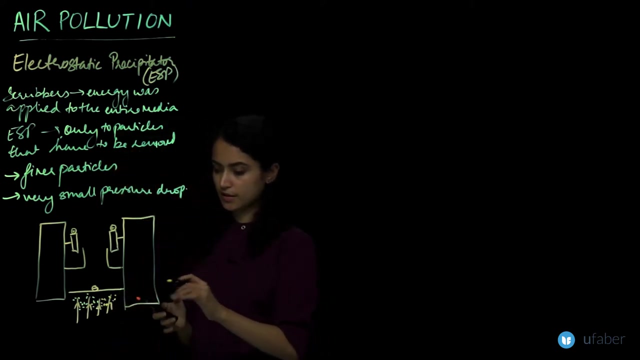 understand. So what I am drawing is a top view. Now, this is not Okay necessarily how all precipitators look, but this is just to give you an idea of what happens. so picture the gas coming in here and it has many particles in it, yes, so what is? 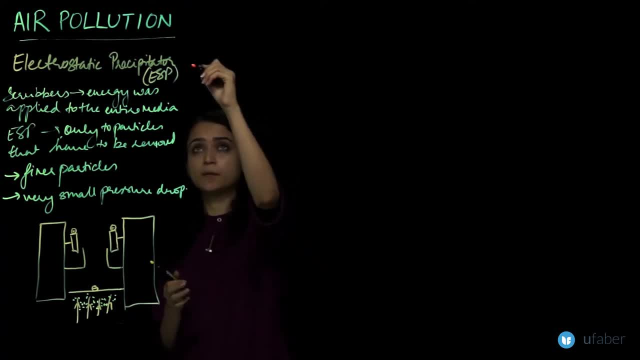 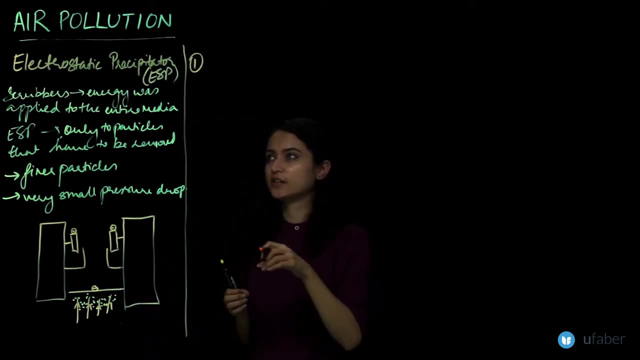 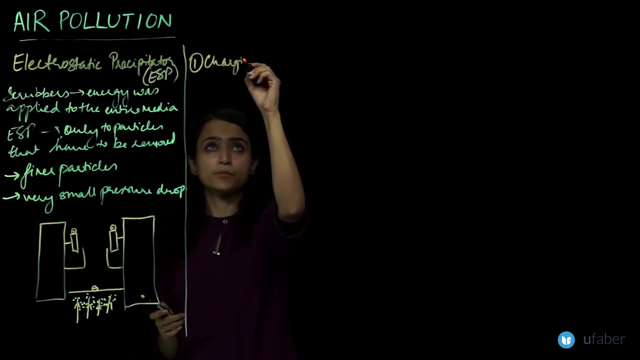 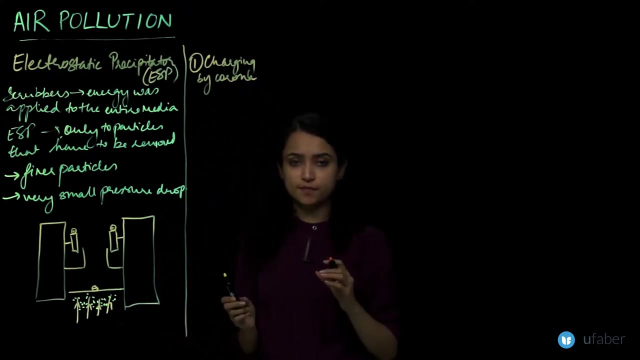 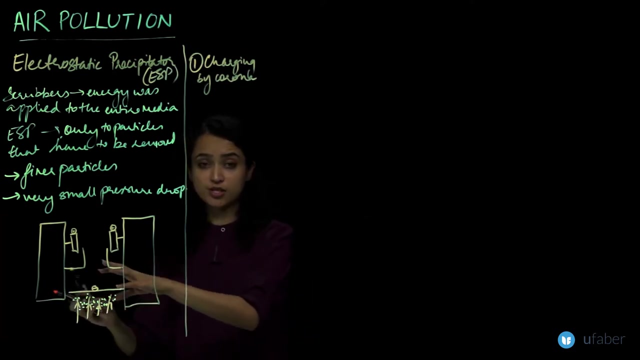 going to happen? is that the first step? yes, so the first step we have in an ESP is the charging of these particles, so the charging by corona discharge. so what will happen is that when these particles, when so the corona discharge creates some ions, and what is going to happen is these particles 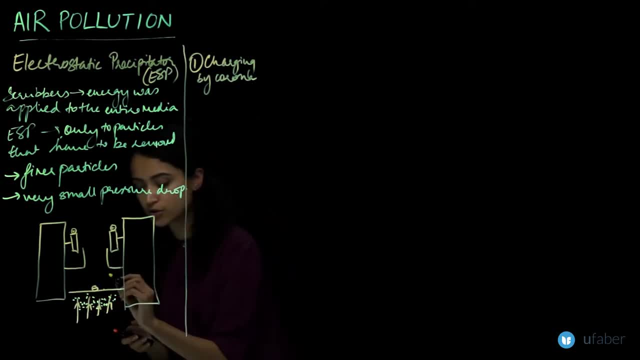 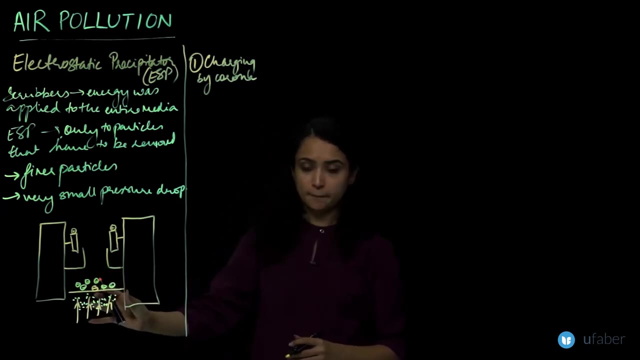 so this is a negative corona discharge that I've drawn here. So what is going to happen is all these particles will also have a negative charge when they come in contact. not in contact, but in the field of this charging electrode. So the charging like I've drawn in the diagram, 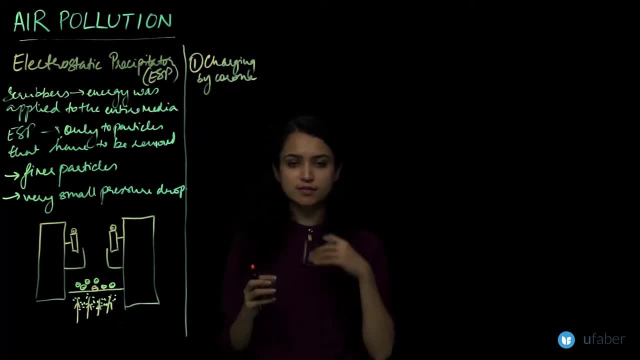 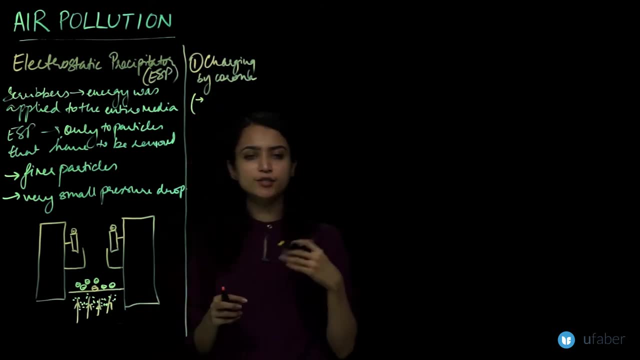 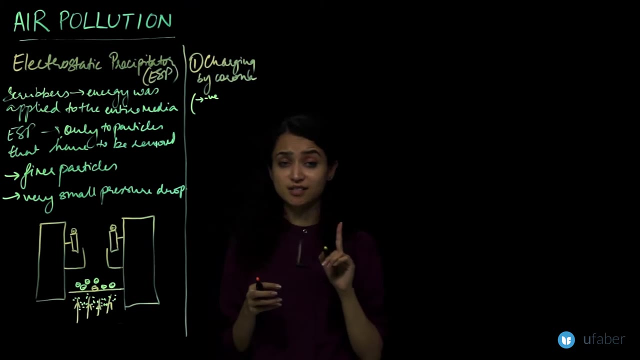 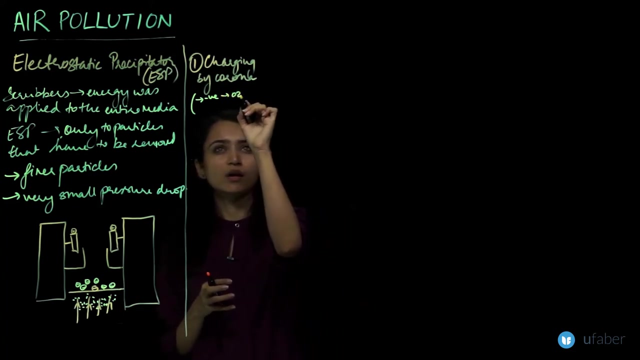 is not necessarily negative, but it is mostly taken as negative. So in the large scale electrostatic precipitators the corona discharge is always negative. and the negative corona discharge has a disadvantage that it leads to the production of a lot of ozone And as 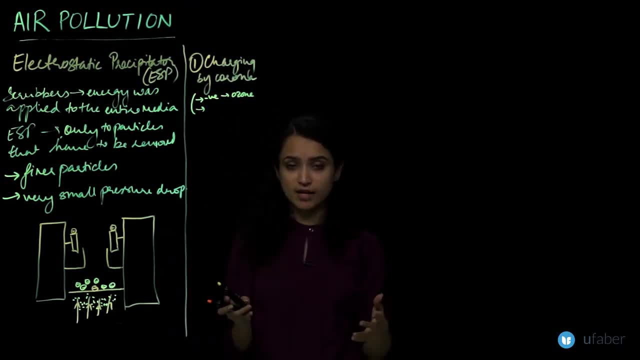 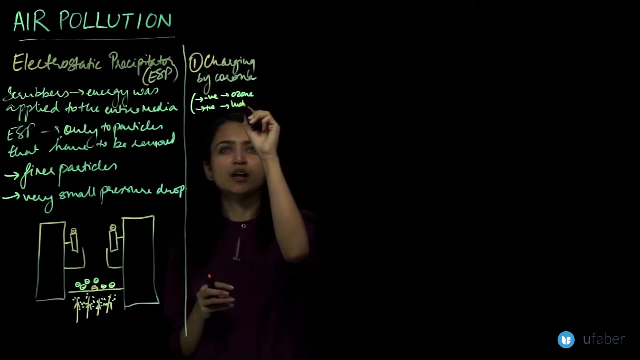 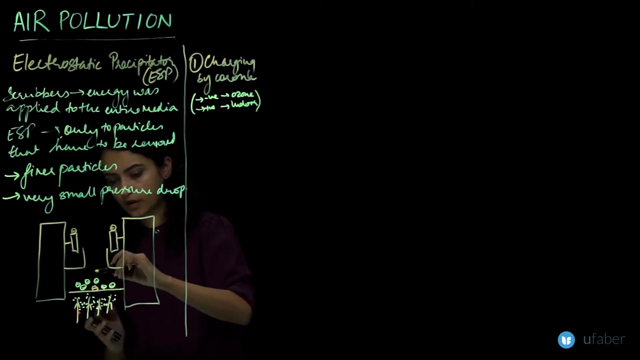 we studied that ground level discharge is always negative. So negative ozone is very harmful and it is a pollutant- in fact it is one of the criteria pollutants- while the positive discharge requires less energy and is usually used in indoor settings. So once these particles are charged, they are going to move in this electrical 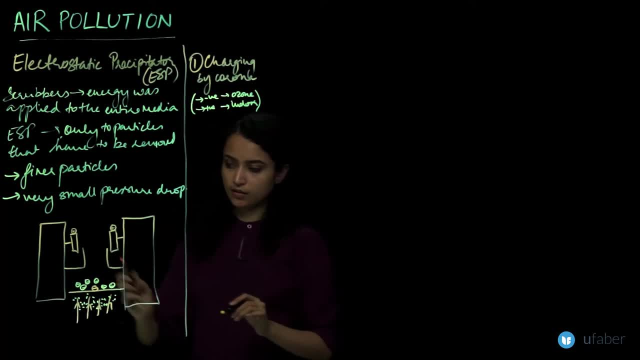 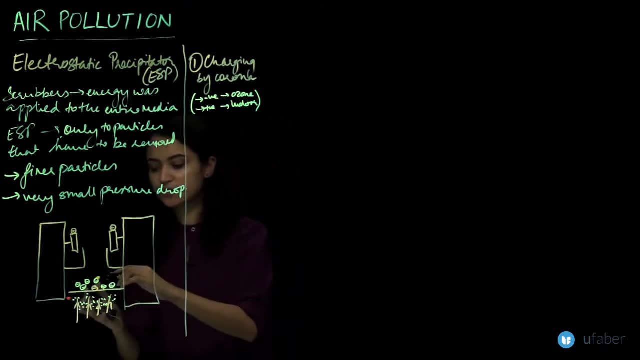 field. so these are our collecting electrodes, the ones that I have marked with a positive. so the there is an electric field that is created and these negatively charged particles are going to move along that field and they will be attracted to these positively charged electrodes. so the second step is: 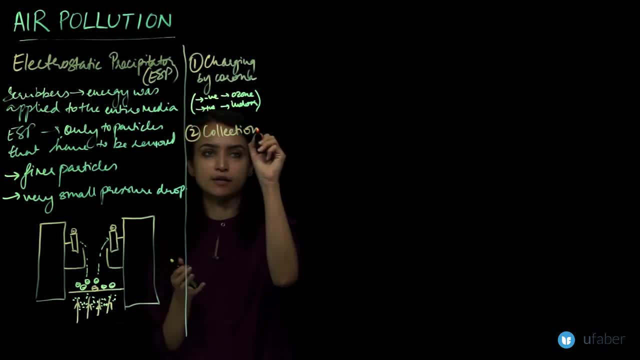 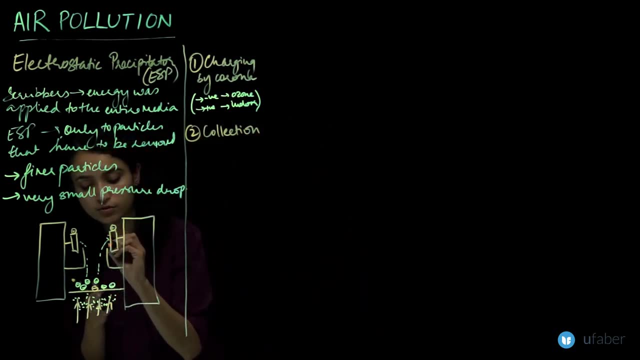 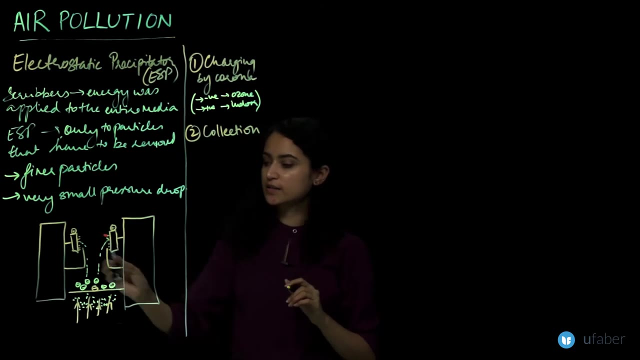 collection of these particles. now these particles are going to come up here and they're all just marking them with little lines to show that they're negative. so what is going to happen is that they are all going to come and deposit here at the collection electrode. so the force is responsible for the 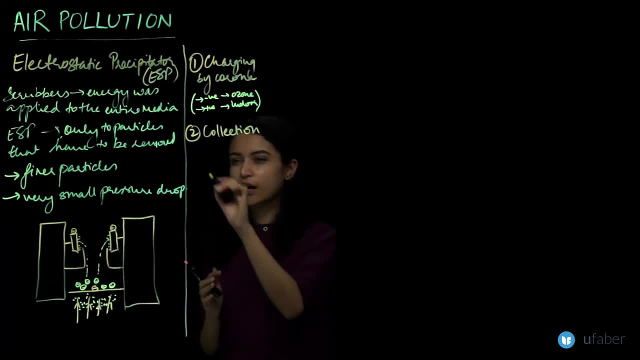 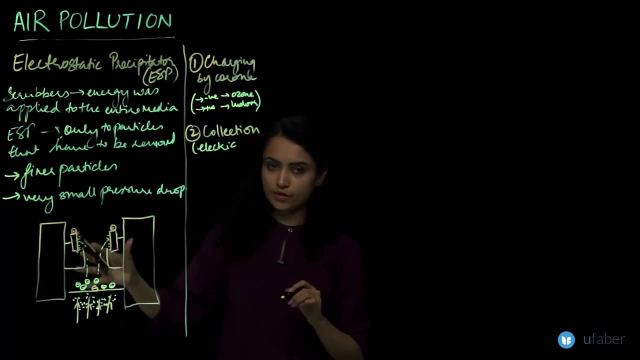 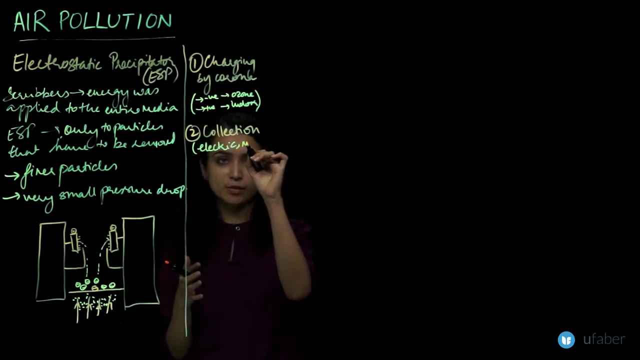 deposition of the particle at the collection electrode are not just electrical, which is pretty obvious from the electric field that is created and the name electrostatic precipitator. so the forces are not just electric, but there would also be mechanical forces in terms of the inertia of the particles, and there are also going to be molecular forces. so 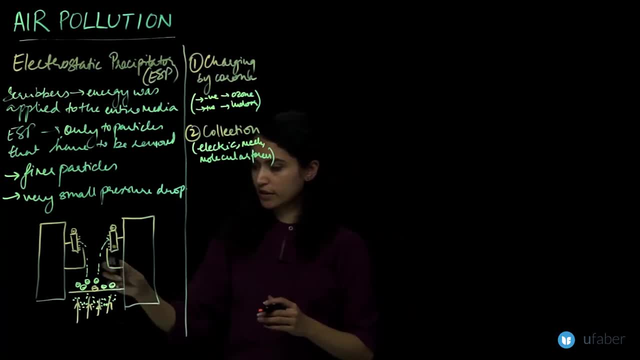 there will come a point where the electric field is going to be electrostatic, precisely theб Smetana fomf, a point where the particles will keep depositing, and they could perhaps deposit in layers well each other, because once they come in contact with this positive electrode, they are going to be positively charged. 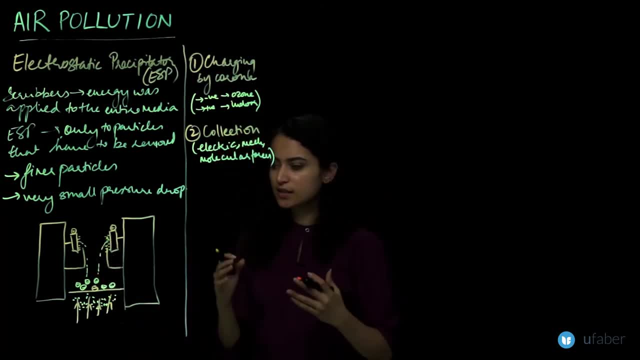 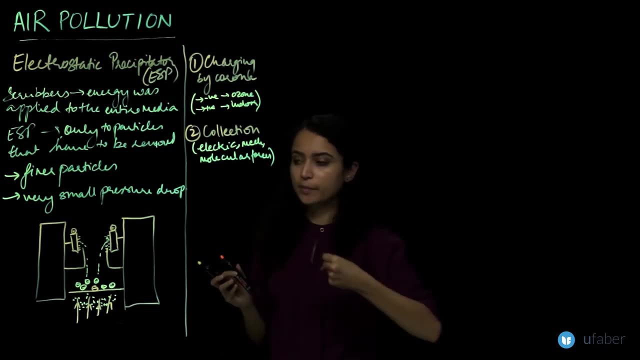 so there could be some layers, a few layers of particles being deposited till, ahh, few layers of particles being deposited till no more particles can be deposited on top of it. so there will be no more like it, no more holding bar in the collecting electrodes to go out the Eye. Ummy, low attention onissors for a lassness of particles now may capture more particles before capturing any energy. 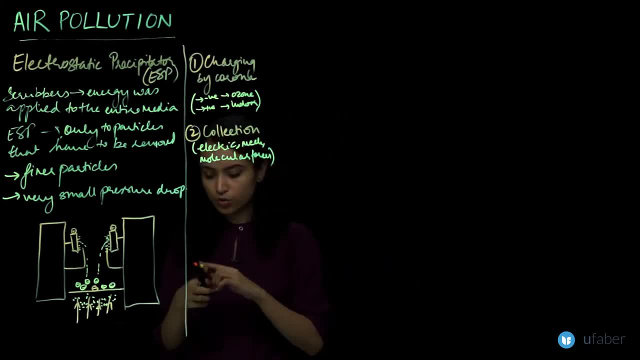 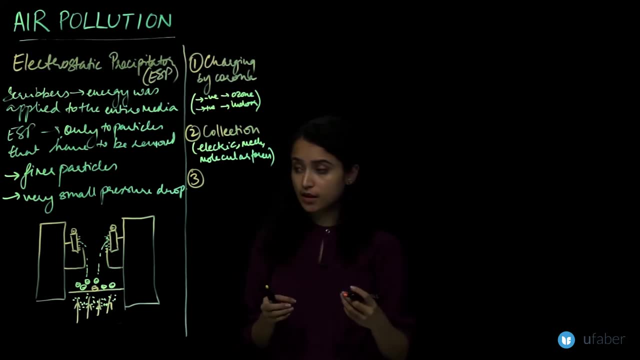 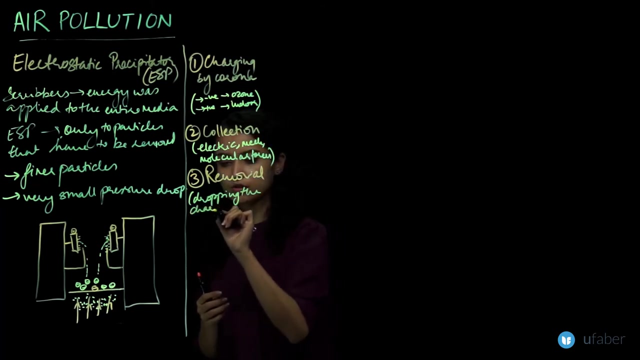 So they are kind of saturated at that point. so what happens at that point is removal of these particles. So there are two ways of removal of these particles. they can either be removed by just quickly, you know, dropping the charge, which is, you know, if you just quickly, momentarily, 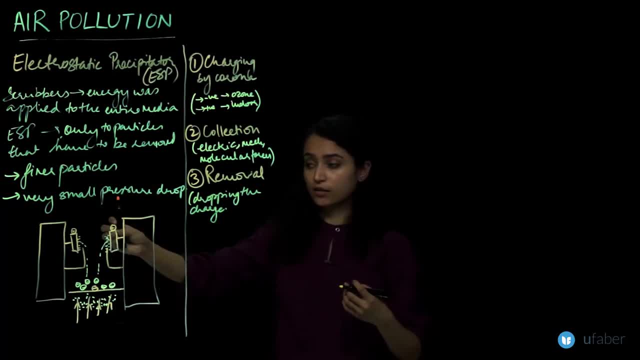 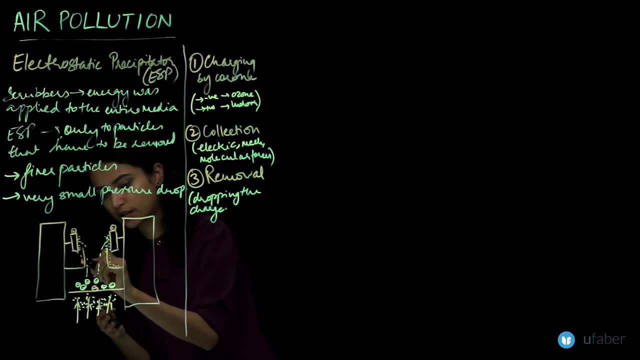 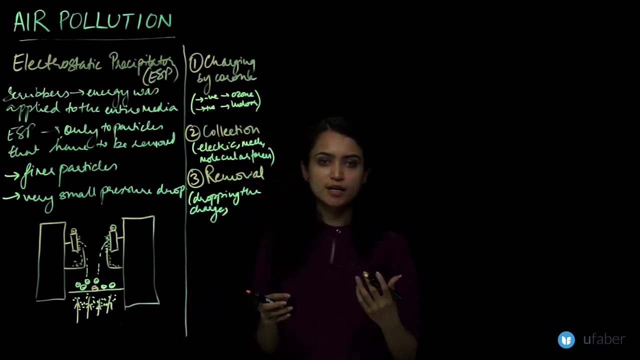 just even momentarily, just turn off the electrodes, all of the particles that are stuck to it will drop off and will collect in a collector here, and if not that then the other process is. So this is simply knocking where. what happens is these collecting plates are actually physically. 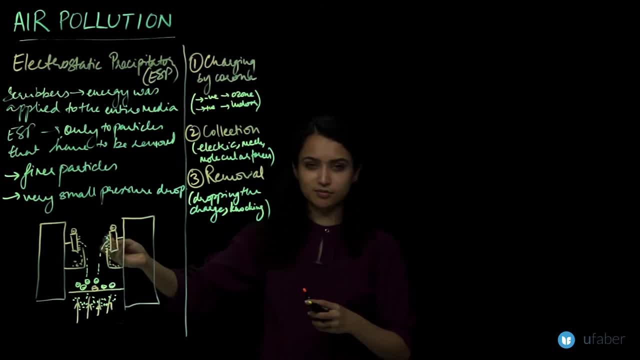 knocked against by another device, another device or something. so say, these plate comes, this plate comes up and knocks against it. so what it is going to do is it is going to loosen all the particles and they are all going to drop and collect here again. 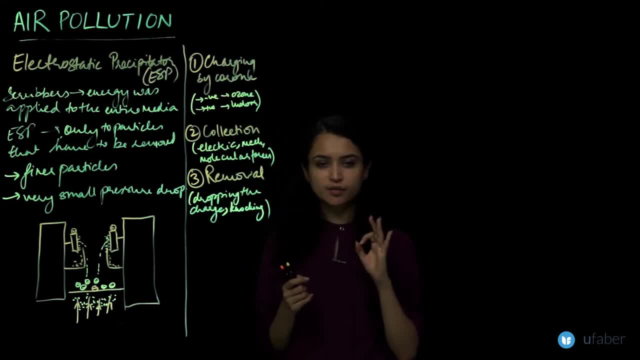 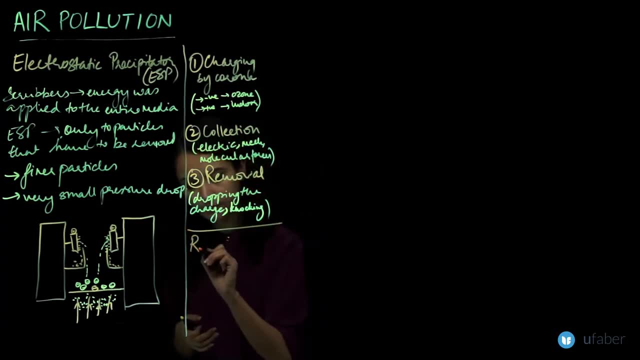 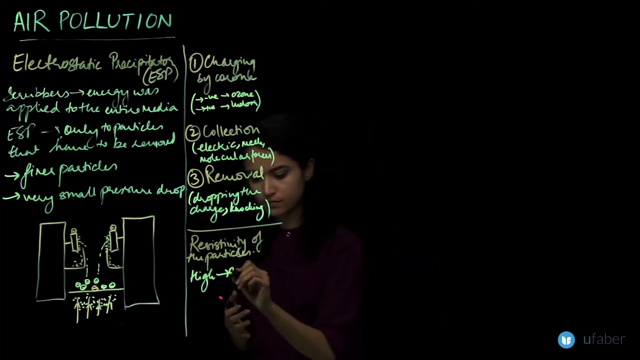 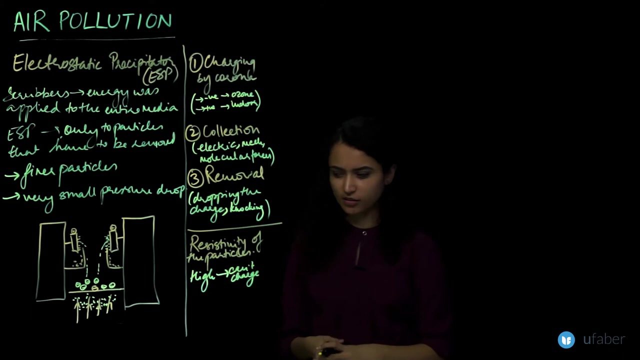 So an important criteria before deciding whether or not you want to remove these particles is the resistivity of the particles. if the resistivity is too high, it would just mean that the particles cannot get charged so easily, Which basically just fails the purpose of an electrostatic precipitator. 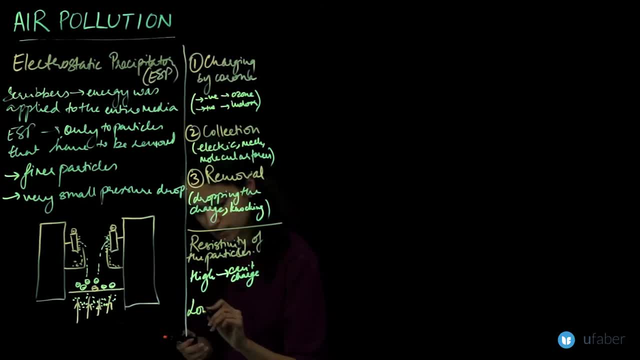 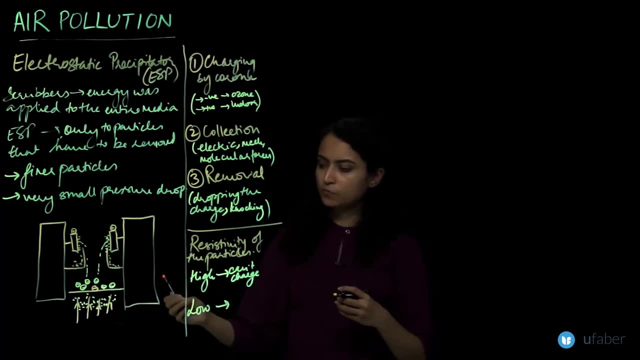 But if they like, if it is too low, the resistivity is if it is too low. what is going to happen is that, as it is moving through the electrical field and when it comes here, the charge, the particle is instantly going to lose its charge and therefore it cannot maintain its charge. 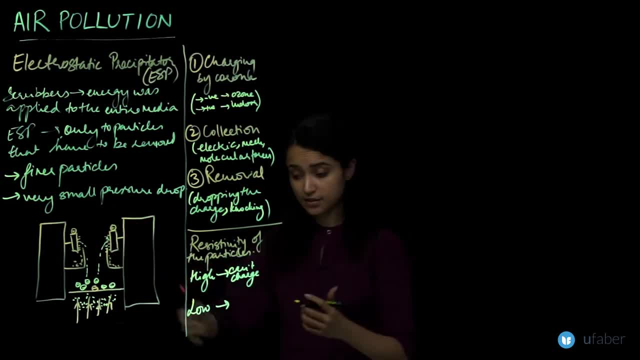 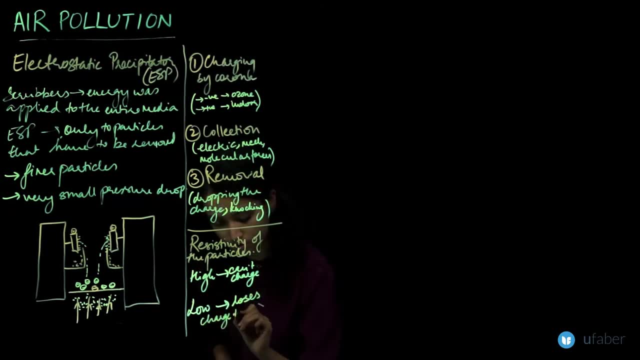 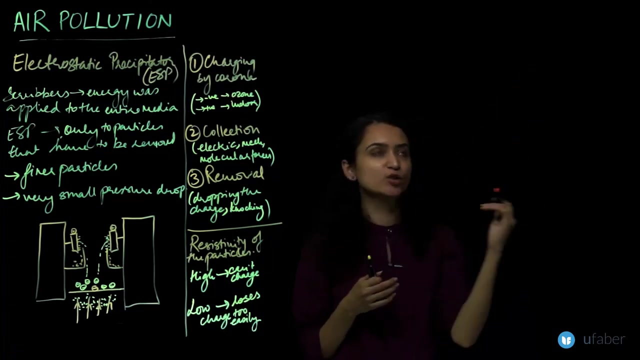 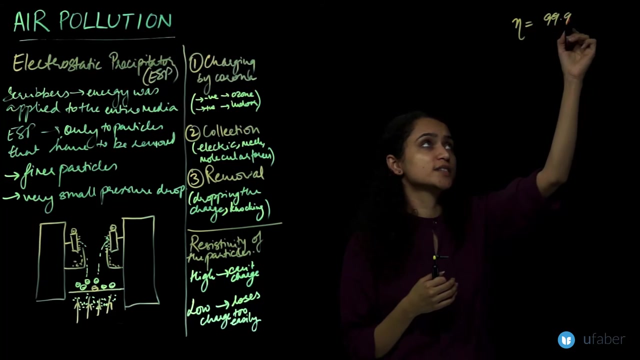 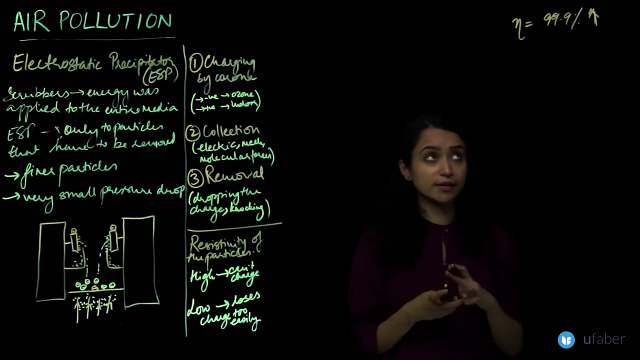 for too long and therefore it will not stick to the plate, so it loses charge too easily. Now coming to some advantages of precipitators. the main advantage why it is widely used is that it has a very high efficiency. The efficiency is mostly 99.9% and up in almost all practical applications. 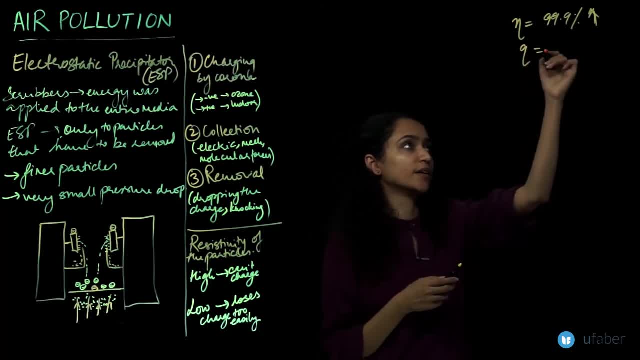 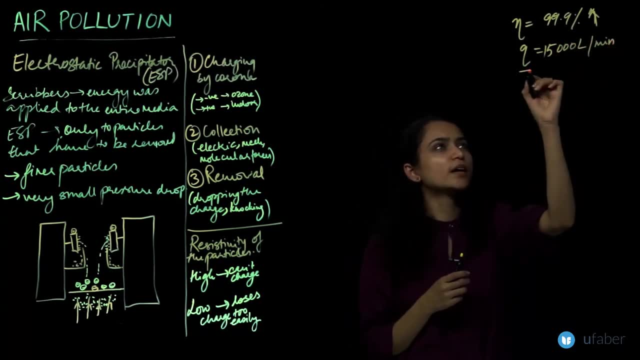 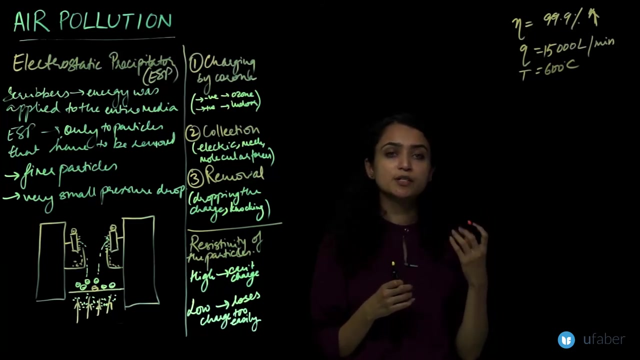 It can handle very high flow rates, at around 15,000 liters per minute. It can handle very high temperatures, so you know you can have a hot gas directly coming into an electrostatic precipitator. The thing is, electrostatic precipitators can also work in a wet environment, so they can. 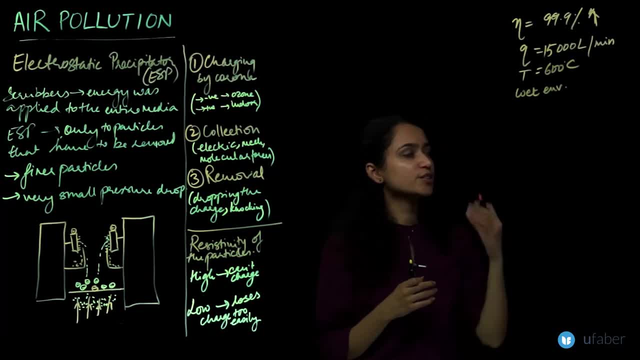 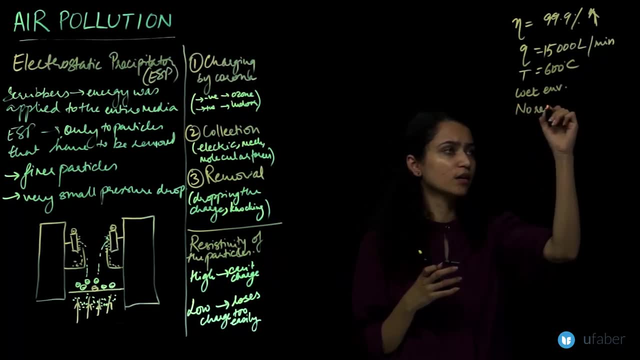 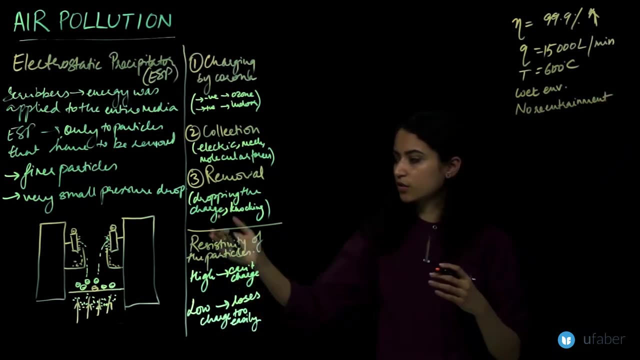 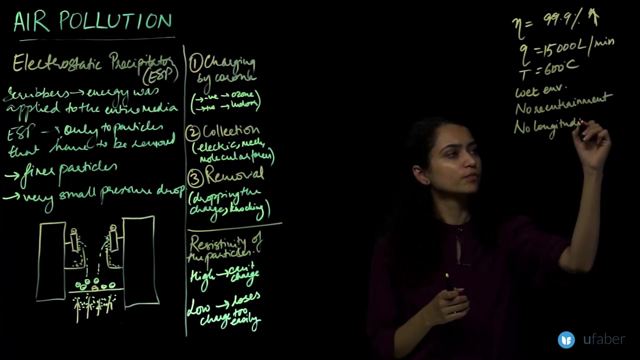 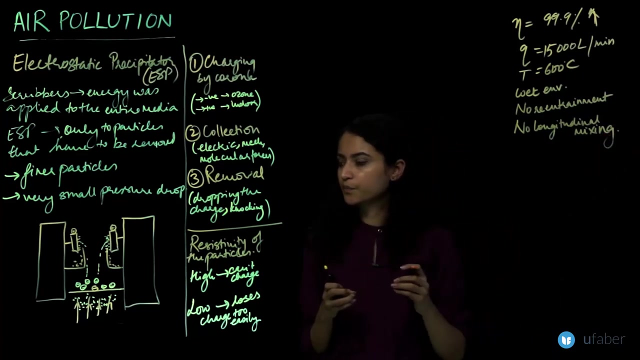 also be used in a wet environment. Electrostatic precipitators: there is no scope for reentrainment and there is no longitudinal mixing. And yes, there is no longitudinal mixing. So an equation which gives us the efficiency of an electrostatic precipitator. I am just 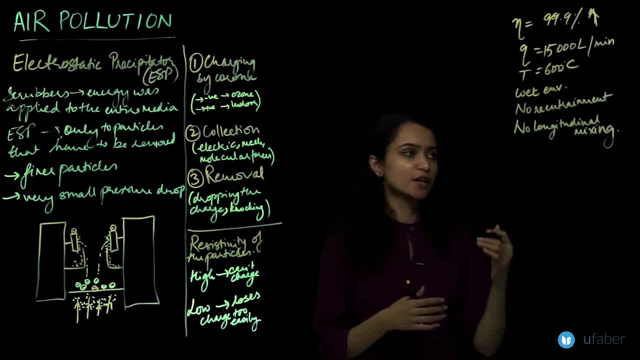 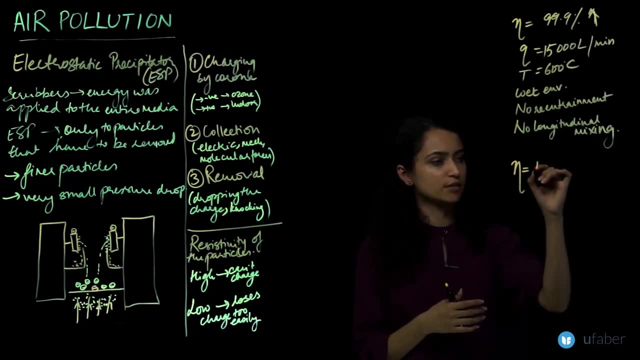 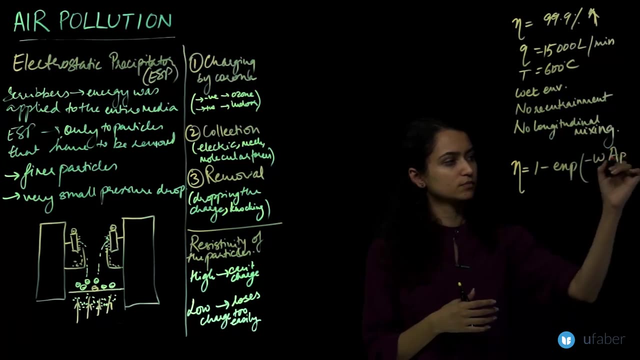 going to introduce one that I am not going to get into how it is derived. So the efficiency of an electrostatic precipitator is 1 minus. so here w is the velocity of the particles, and I am not going to get into how it is derived. I am not going to get into how it is derived. 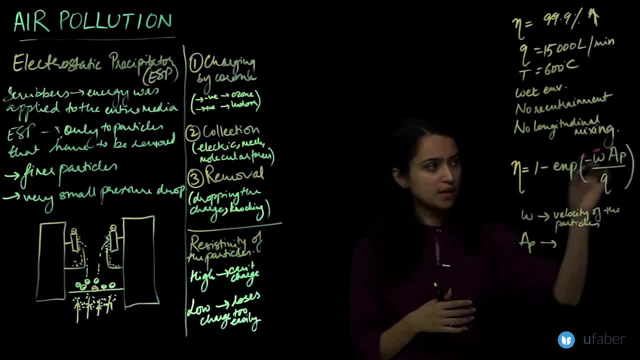